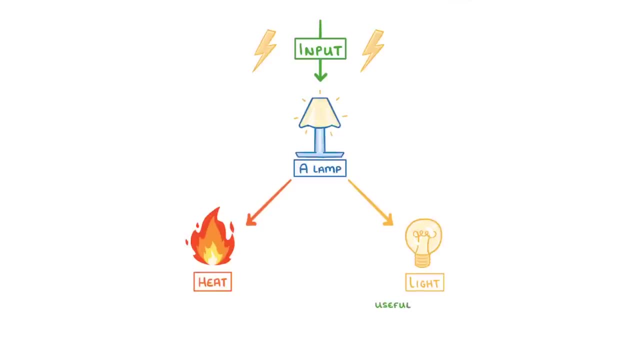 is to provide light, we consider the light energy as useful energy output, whereas the heat energy can be classed as wasted energy or non-useful energy output. The efficiency of a device like this is just the proportion of the energy supplied, so the input energy that's actually transferred into the useful energy output. 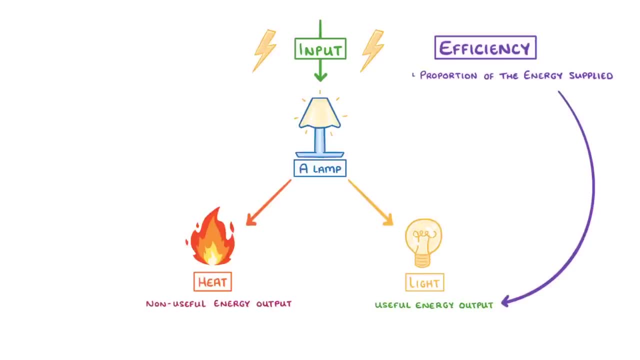 so transferred into light energy. When it comes to your exams, you'll need to be able to calculate the efficiency of a device as a decimal or a percentage, by using the equation which is: efficiency equals useful energy output divided by the total energy input. Or, if you're, 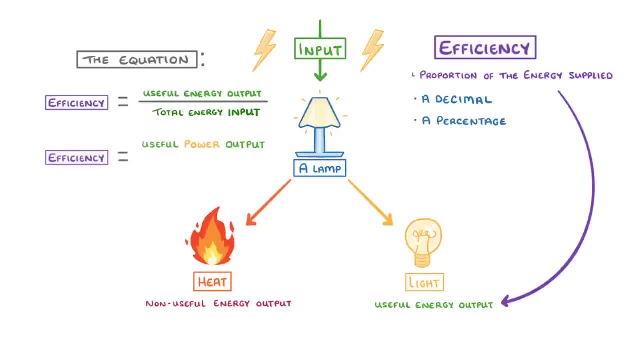 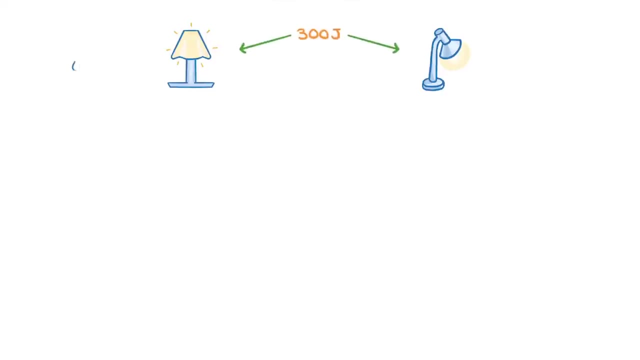 using power, then its efficiency equals useful power output. To put this into practice, let's imagine that we have two lamps and we supply 300 Joules to each of them. The one on the left has an old incandescent bulb which converts 45 Joules. 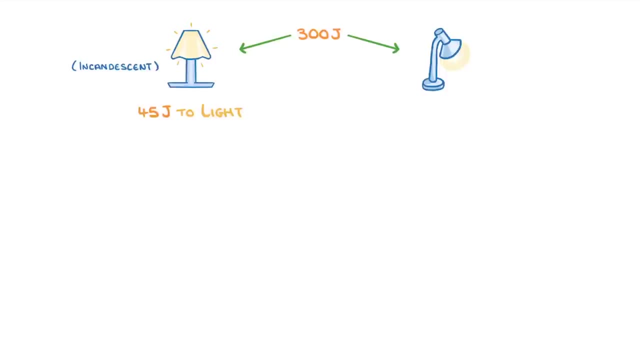 of that, 300 into light energy. Meanwhile, the other one has a modern LED bulb which converts 225 Joules into light. How many times more efficient is this than the other? If you're more efficient, then the LED lamp is more efficient. 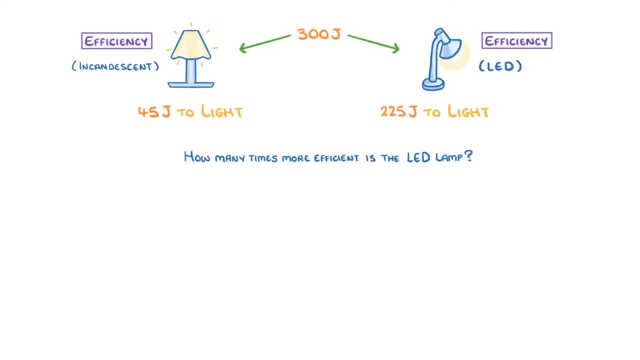 First of all, we need to calculate the efficiency of each bulb. For the incandescent bulb, we would do 45 Joules, which was the useful output, divided by 300 Joules, which was the total input. This gives an efficiency of 0.15.. Meanwhile, for the LED, we do 225, divided by 300, to 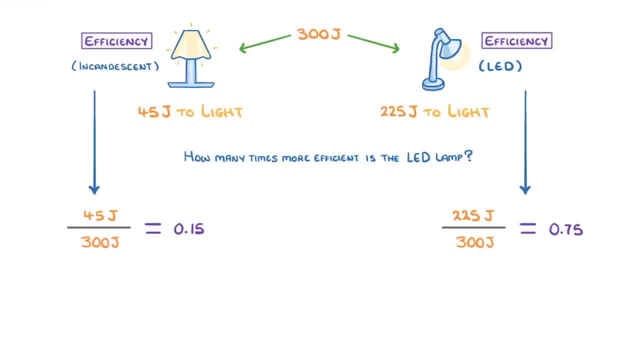 get an efficiency of 0.75.. Then to find out how many times more efficient the LED lamp is, we just divide its efficiency of 0.75, by the efficiency of the incandescent bulb, 0.15, which gives us 5.. So the LED lamp 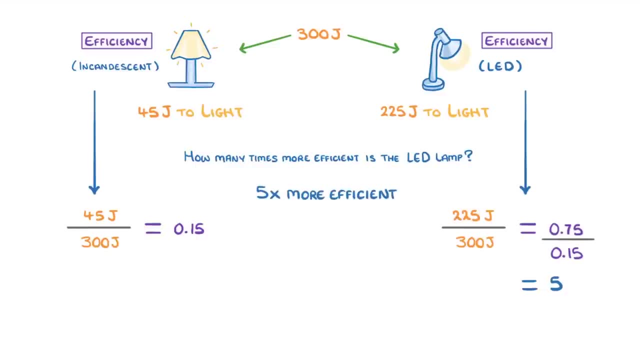 is 5 times more efficient. If we instead wanted these efficiency figures in percentage terms, we would just multiply them by 100,, giving us 15% and 75%, And we could then do similar things. We could then multiply them by 100,, giving us 15% and 75%, and we could then do similar things.